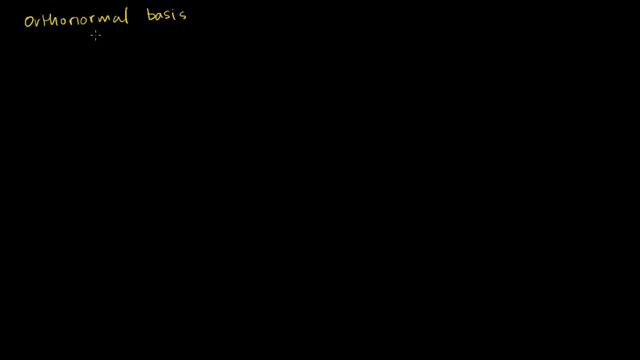 We know what an orthonormal basis is, but the next obvious question is: what are they good for? And one of the many answers to that question is that they make for good coordinate systems or good coordinate bases, For example the standard basis or the standard. 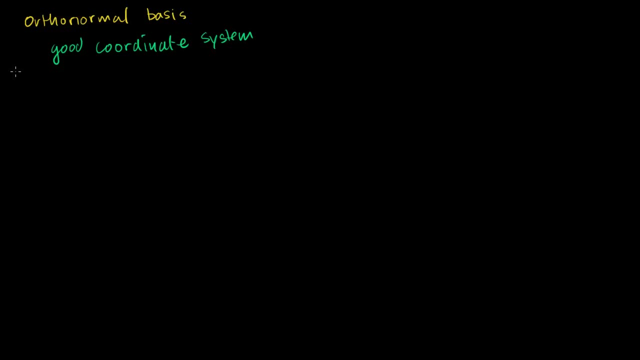 coordinates. let me write the standard basis in Rn. So if we're dealing with Rn, so the standard basis for Rn is equal to. well, I could write it as E1,, E2, and all of that, but I'll actually write out the vectors. 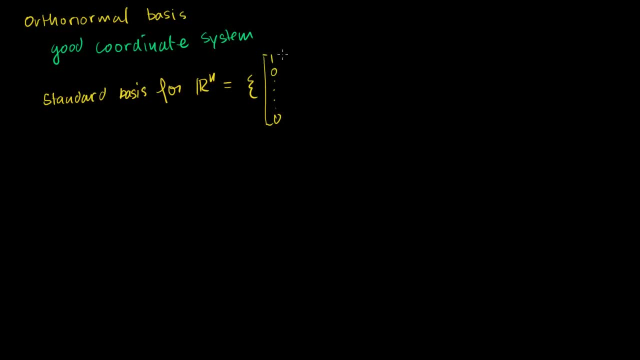 E1 is just 1, with a bunch of 0's all the way. E2, and this is going to be n? 0's right there. E2 is going to be 0.. 1, with a bunch of 0's all the way. 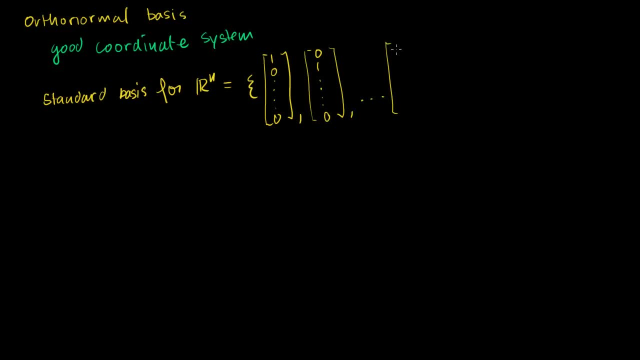 And then you're going to go all the way to En, which is going to have a bunch of 0's, and then you're going to have a 1.. The standard basis that we've been dealing with throughout this playlist is an orthonormal set is an. 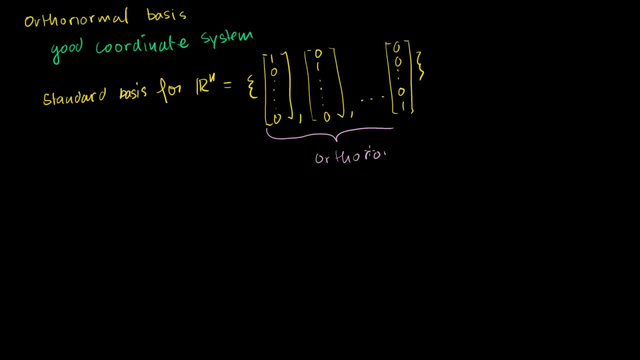 orthonormal basis. It's an orthonormal basis. Clearly, the length of any of these guys is 1.. If you were to take this guy dotted with the other guys with yourself, you're going to get 1 times 1. 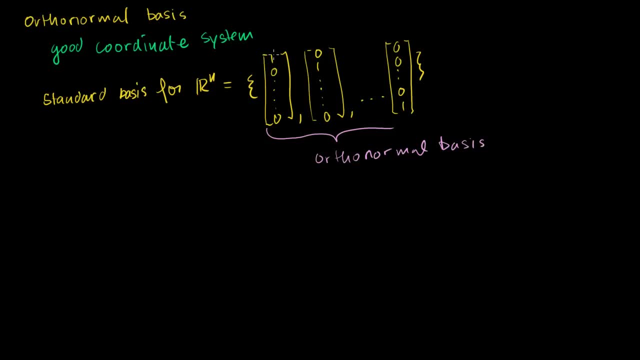 plus a bunch of 0's times each other, so it's going to be 1 squared. so it's going to be 1.. And that's true of any of these guys And clearly they're orthogonal. You take the dot product of any of these guys with any of the. 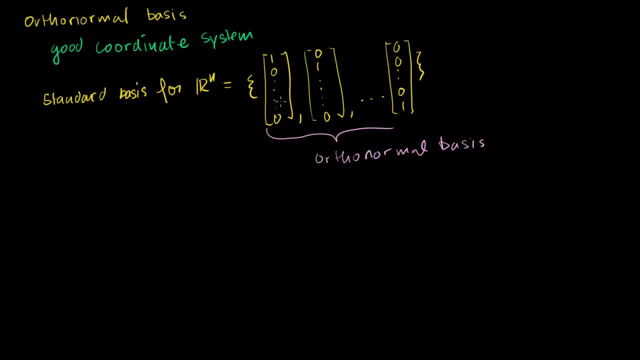 other ones. you're going to get a 1 times 0, and a 1 times a 0, and then a bunch of 0's. so you're going to get 0's. So they're clearly each have lengths of 1, and they're all. 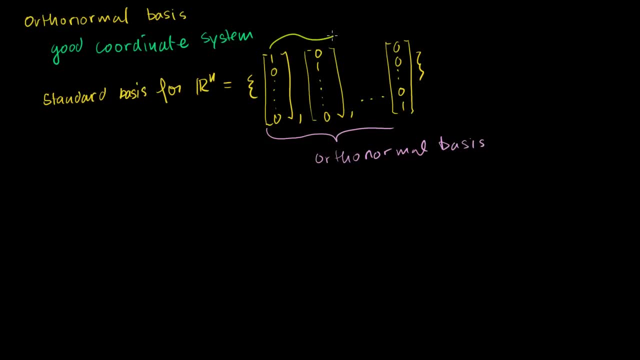 orthogonal And clearly this is a good coordinate system. But what about other orthonormal basis? Obviously, this is one specific example. I need to show you that all orthonormal bases make for good coordinate systems. So let's say, I have some set, some orthonormal set of 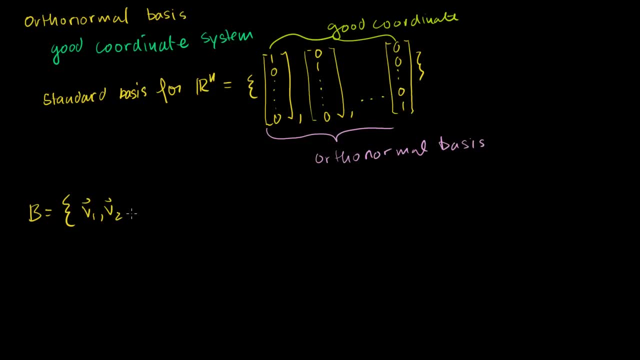 vectors. so this is v1, v2, all the way to vk And it is an orthonormal basis, Orthonormal basis for some subspace v And this is a k-dimensional subspace because you have k basis vectors in your basis. 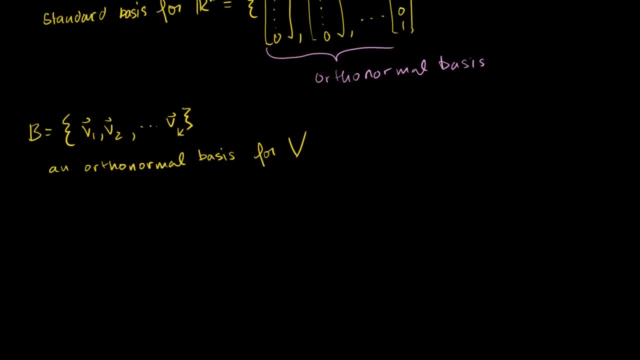 Now let's experiment with this a little bit. I'm claiming that this would make that the coordinate system with respect to this is good. But what does it mean to be good? I mean, the standard basis is good, But that's just because we use it and it seems to be easy to. 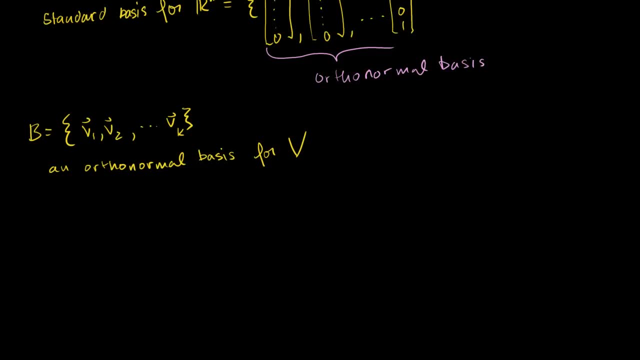 deal with. But let's see what I. when I say good in this context, what do I mean? So let's experiment. If I say that some vector x is a member of v, that means that x can be represented as a linear combination of these. 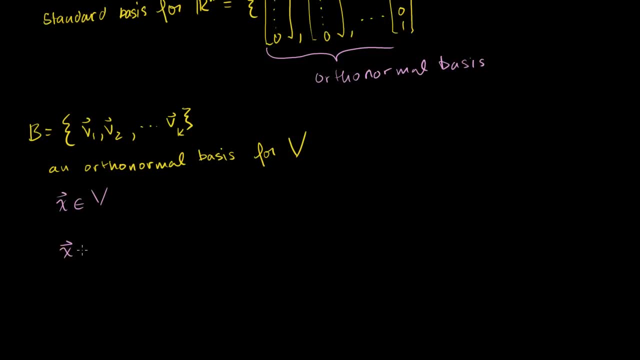 characters up here. So x can be represented as some constant times v1 plus some constant times v2.. Plus you know The ith constant times vi all the way, if you just keep going all the way to the kth constant times vk. 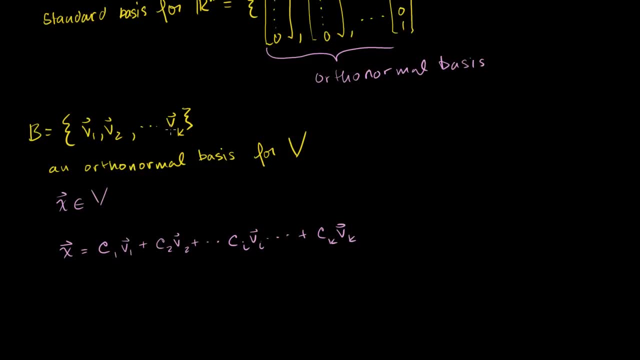 That's what being a member of the subspace means. The subspace is spanned by these guys, so this guy can be represented as a linear combination of those guys. Now, what happens if we take the dot product of both sides of this equation with vi? 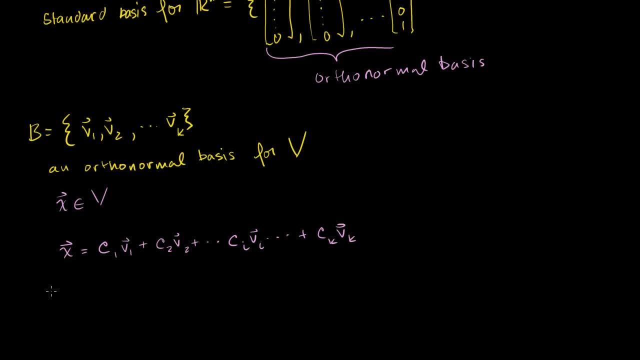 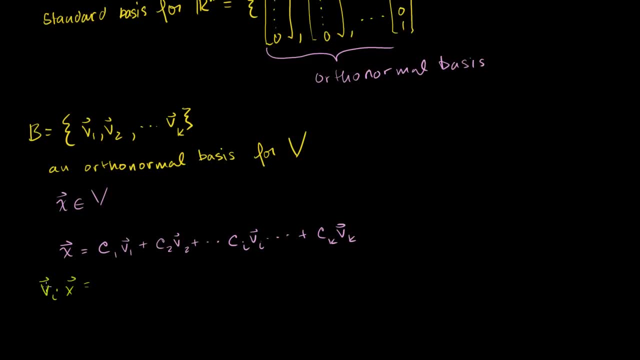 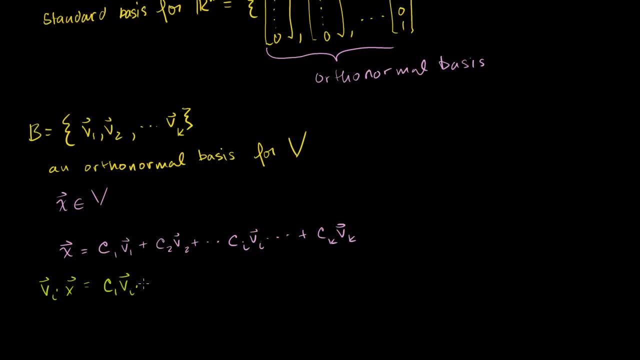 out. it's going to be c1 times vi dot v1, plus c2 times vi dot v2, plus all the way to ci times vi dot vi, And then you keep going plus all the way to ck times vi dot vk. Now, this is an orthonormal set. 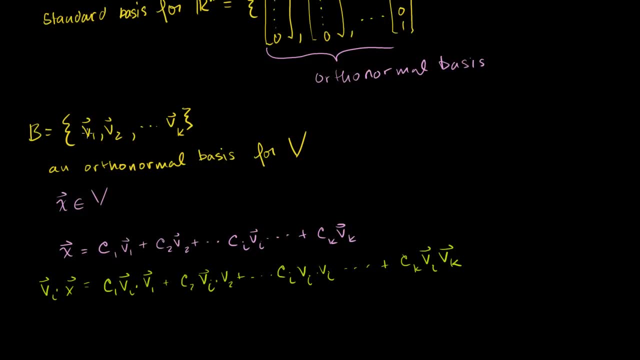 That means, if I take two vectors that are different than each other in our basis right here, that if you take their dot product you're going to get 0. They're orthogonal to each other. So these are two different vectors in our set. 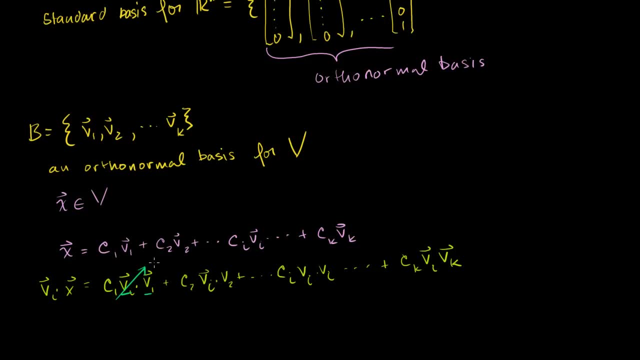 They're going to be orthogonal, so this term is going to be 0.. It's going to be 0 times c1, so it's going to be 0.. This term is also going to be 0, assuming that i isn't 2.. 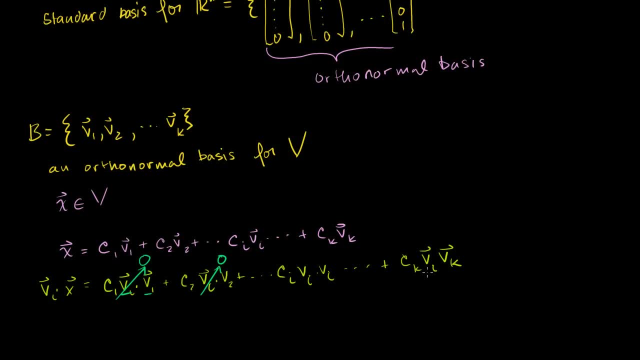 Let's just assume that This term over here, let's assume that i isn't k, It's also going to be equal to 0.. So all of the terms are going to be 0, except for the case where vi is equal to well- in this case, vi- except for the. 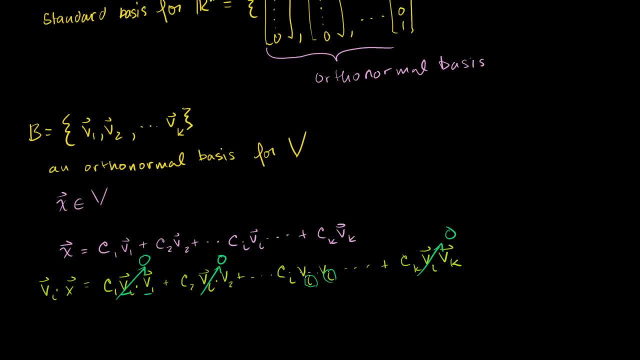 case where this subscript is equal to that subscript. And then what is vi dot vi? Well, this is orthonormal, has two parts, They're orthogonal to each other and they're each normalized, Or they each have length 1.. 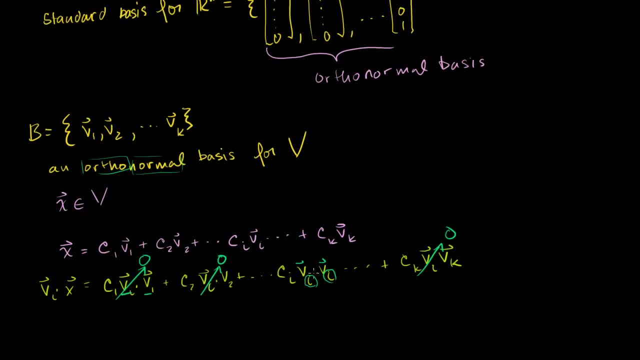 so vi dot, vi dot with vi is going to be equal to 1.. So this whole equation is simplified to v sub i, which is one of these guys- it's the ith member of our basis. set dot x where x is just any member of the. 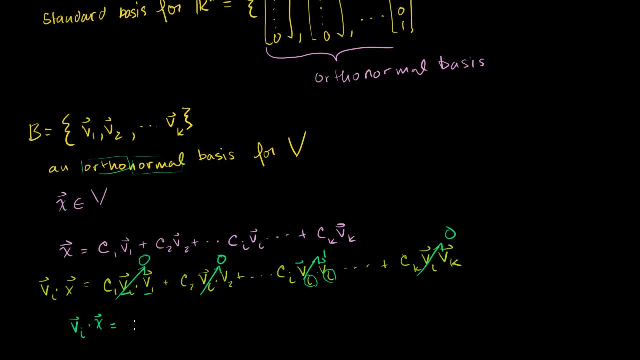 subspace is equal to. the only thing that's left over is 1 times ci, So it's just equal to ci. Now, why is this useful? We were just experimenting around and we got this nice little result here. Why is this useful in terms of having a coordinate system? 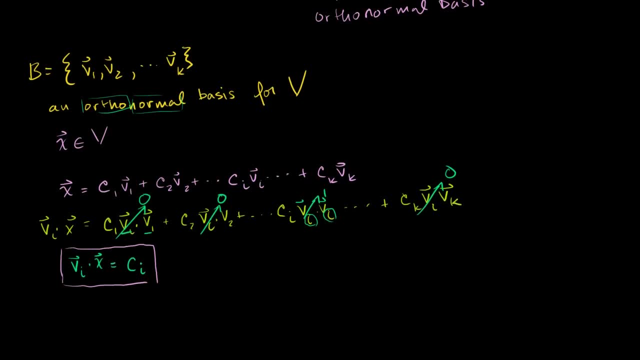 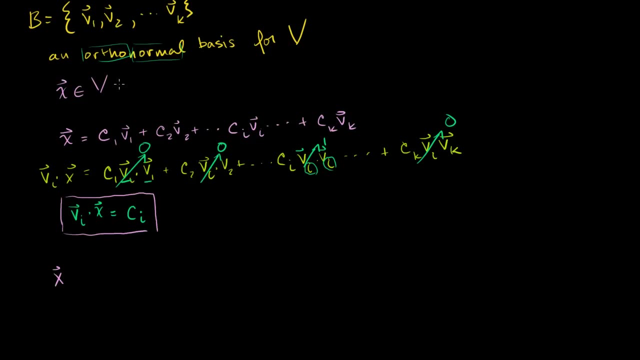 with respect to this basis. So let's remind ourselves what a coordinate system is here. So if we wanted to represent the vector x, which is a member of our subspace, with coordinates that are, with respect to this basis of the subspace, right, 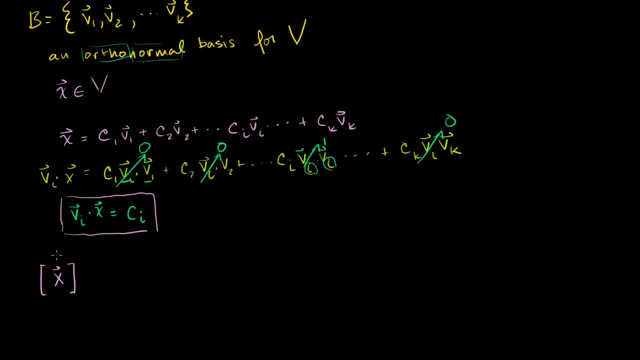 A subspace can have many bases, but this is the basis that we're choosing. So we want to write x with respect to the basis b. What do we do? The coordinates Are going to just be the coefficients on the different basis vectors. 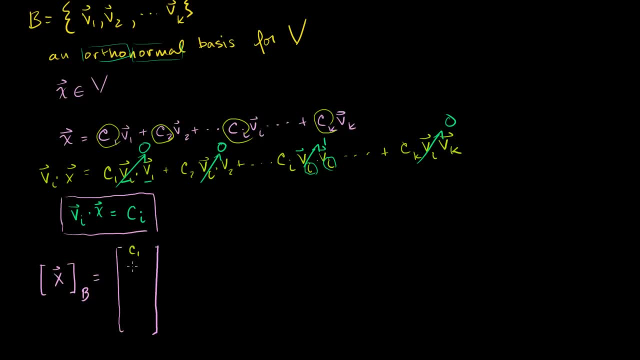 This is all a bit of a review. right, It's going to be c1, c2, you're going to go down to ci and then you're going to go down all the way to ck. You're going to have k terms, because this is a k. 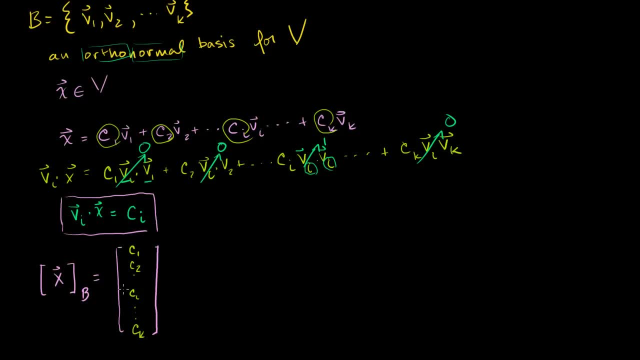 dimensional subspace. Now, normally this is not such an easy thing to figure out. If I give you some vector x- I mean we've seen it before- if you have x represented in a b coordinate system, then you can multiply it times the change of basis matrix and you can. 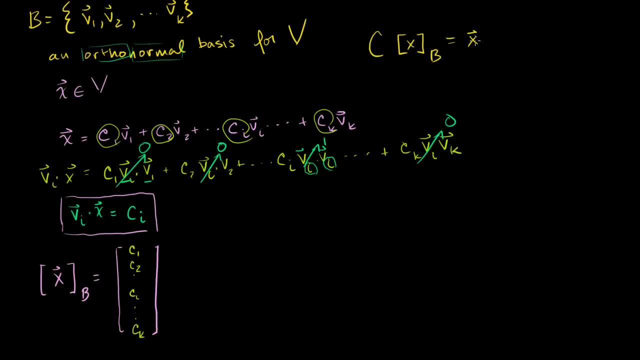 just get regular x. But if you have regular x and you need to find this one, if c is invertible, then you can apply this equation right here, which isn't always the case. This is only if c is invertible. 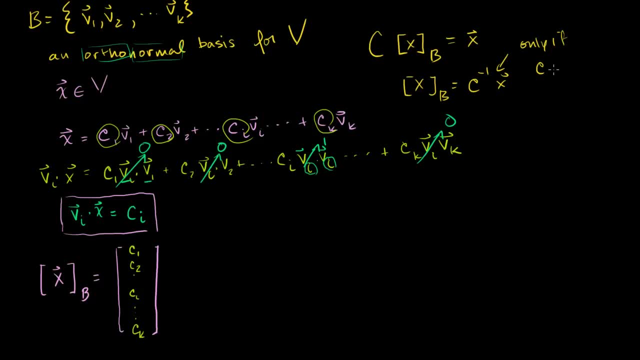 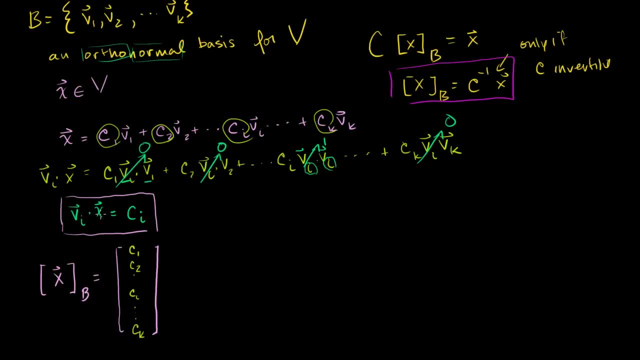 So this is one way that if I give you your x to get your b representation of x, but if c isn't invertible, then you're just going to have to solve this equation. You're going to have something on the right-hand side here. 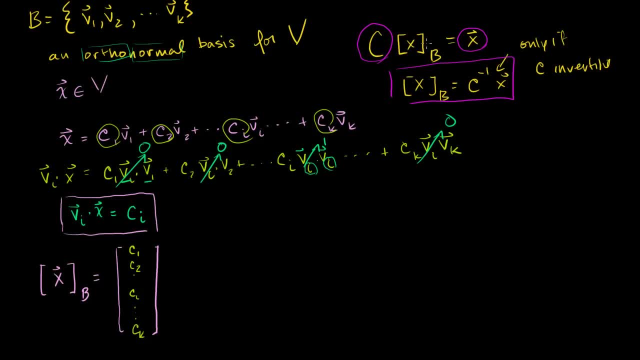 You're going to have a change of basis matrix and then you're going to have to solve that equation. So it's kind of a you know for an arbitrary basis. that can be pretty painful, But what do we have here? 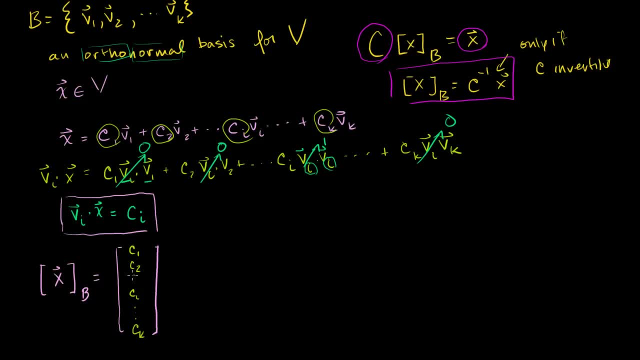 We have a very simple solution for finding the different coordinates of x. So this is the same thing as being equal to. c1 is just going to be equal to my first basis vector dotted with x. right, We say ci is just the i-th basis vector dotted with x. so 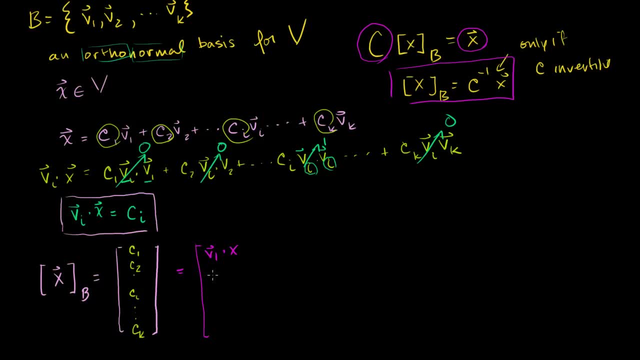 c1 is going to be the first basis vector dotted with x. c2 is going to be my second basis vector dotted with x, And you're going to go all the way down to ck is going to be my k-th basis vector dotted with x. 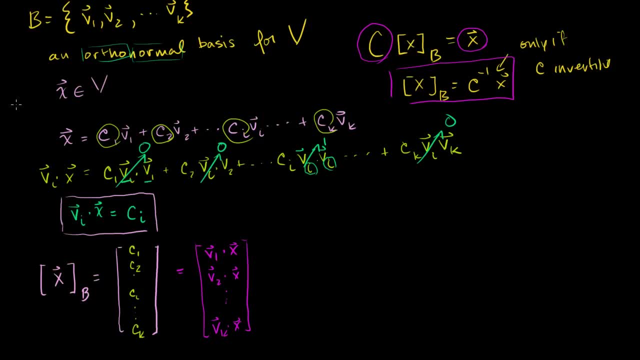 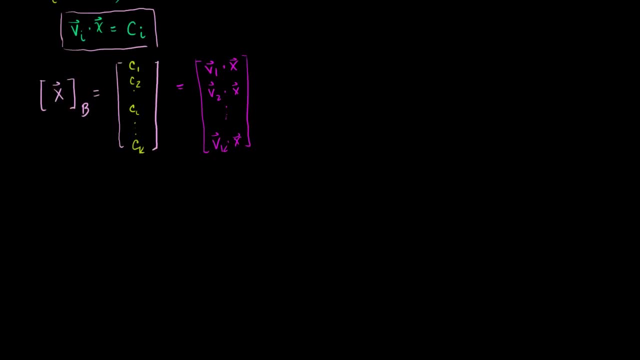 Let me show you that this is actually easier. So let's do a concrete example. So let's say I want to leave this result up here. Let's say that I have two vectors. Let's say that v1 is the vector 3. fifths, 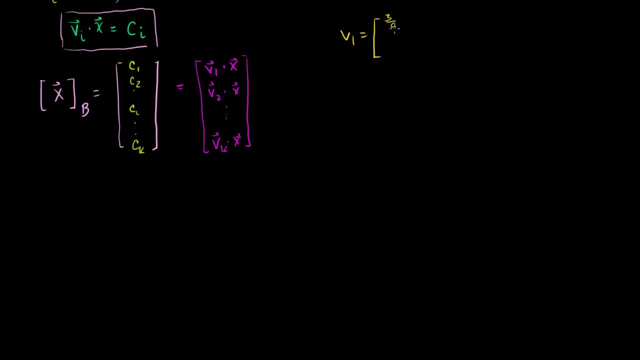 Let me write it this way: Let's say it's 3 over 5 and 4 over 5.. And that v2 is equal to minus 4 fifths, 3 fifths. And let's say that the set B is equal to. it's comprised of: 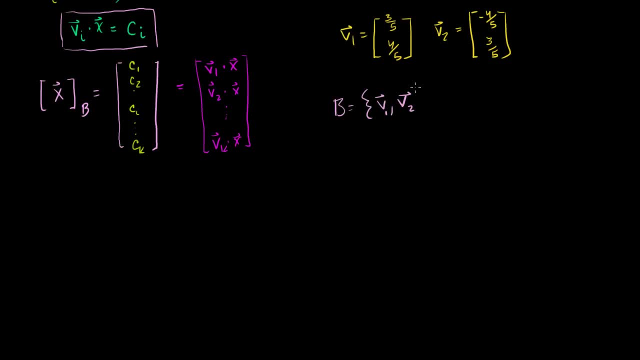 just those two vectors, v1 and v2.. Now I'm claiming, or I'm about to claim, that this is an orthonormal set. Let's just prove it to ourselves. So what is the length of v1 squared? 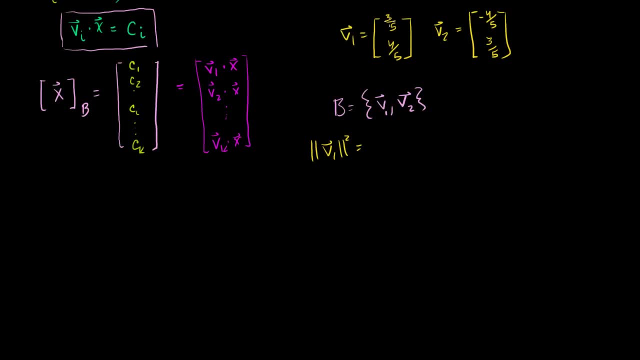 Well, that's just v1 dotted with itself, So that's 3 fifths squared, which is 9 twenty-fifths, plus 4 fifths squared, which is 16 twenty-fifths, which is equal to 25 over 25, which is equal to 1.. 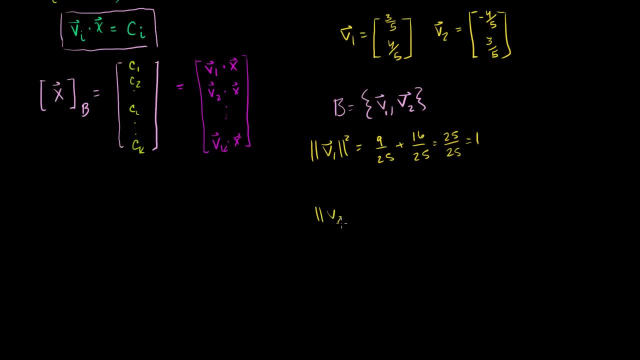 So this guy definitely has length 1.. What is the length of v2?? Well, it's going to be this guy. squared Negative 4 fifths squared is 9 twenty-fifths plus 3, sorry, minus 4 fifths squared is plus 16 twenty-fifths. 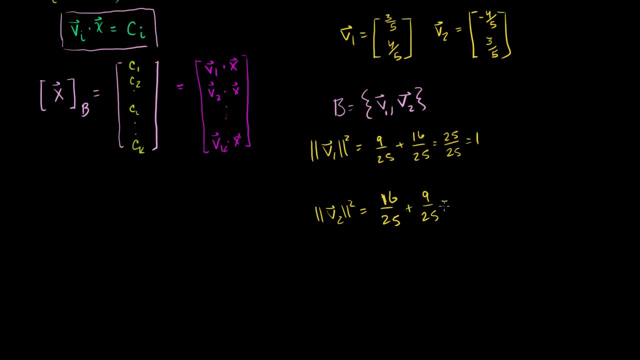 And then 3 fifths squared is 9, twenty-fifths, And once again the length squared is going to be 1, or the length is going to be 1.. So both of these guys definitely have length 1.. And now we just have to verify that they're orthogonal with. 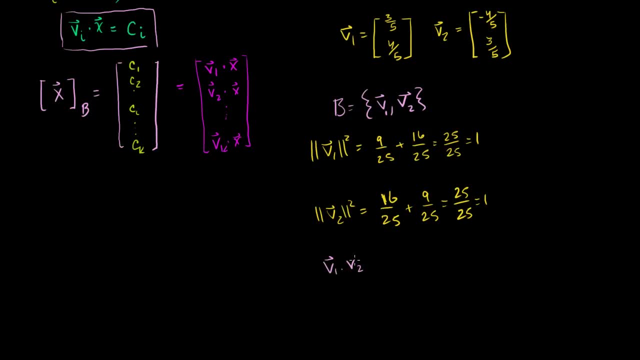 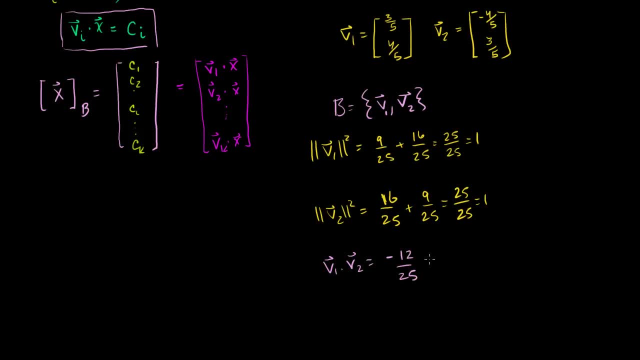 So it's going to be minus 12 twenty-fifths, plus 4 fifths times 3 fifths, which is going to be plus 12 twenty-fifths, which is equal to 0.. So these guys are definitely orthogonal with respect to. 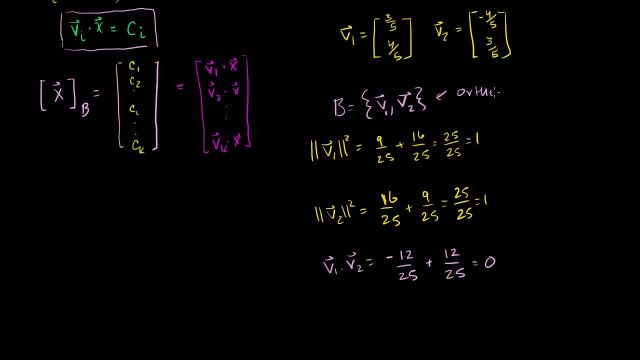 each other and their lengths are 1.. So this is definitely an orthonormal set, And so that also tells us that they're linearly independent. So let's say that my set B is the basis for some subspace v, For some subspace v. 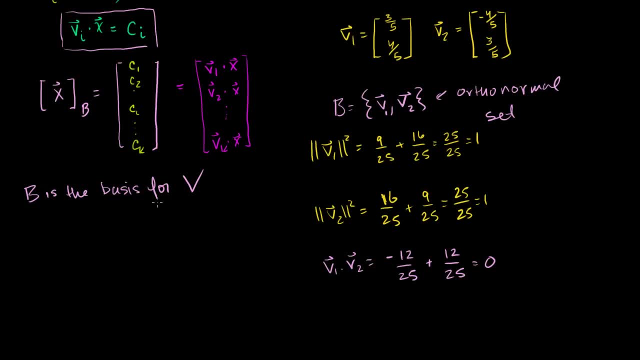 And let's say- and actually it's not a, we don't have to say that it's the basis for R2.. It's a basis for R2.. How do we know it's a basis for R2?? I have two linearly independent v's. 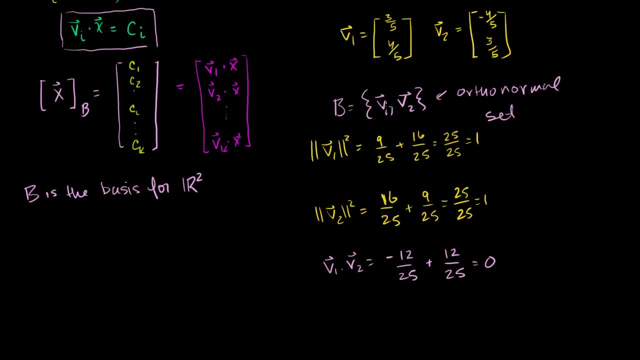 I have two linearly independent vectors in my basis and it's spanning a two-dimensional space- R2, so this can be a basis for all of R2.. Now, given what we've seen already, let's pick some random member of R2.. 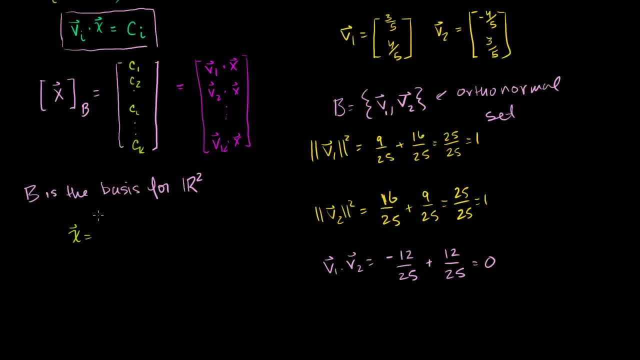 So if we pick some random member of R2, let's say that x is equal to- I don't know, I'm just going to pick some random numbers- 9 and minus 2.. 9 and minus 2. x is equal to- I don't know, I'm just going to pick some. 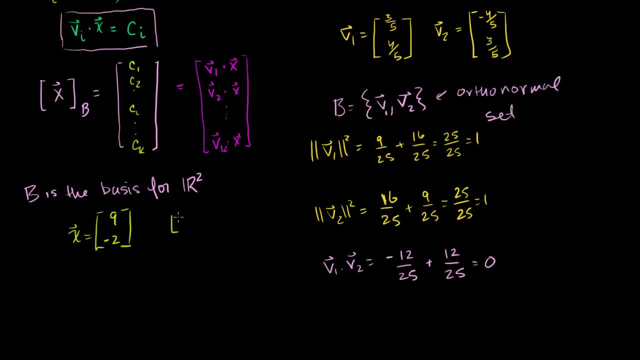 know this was an orthonormal basis and we wanted to figure out x in b's coordinates. what we would have to do is we would have to create the change of basis matrix. So the change of basis matrix would be 3 fifths, 4 fifths. 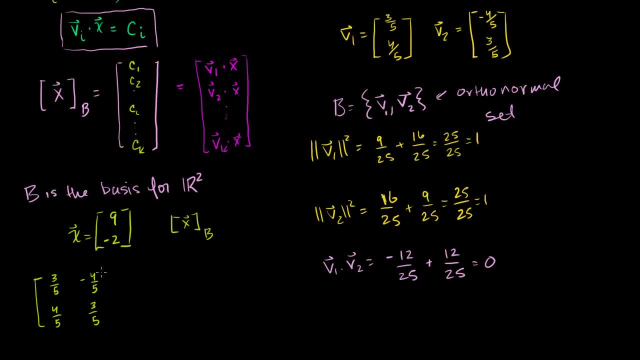 minus 4 fifths and then 3 fifths. We would say that times my b-coordinate representation of x is going to be equal to my regular representation of x or my standard coordinates of x, And I would have to solve this 2 by 2 system. 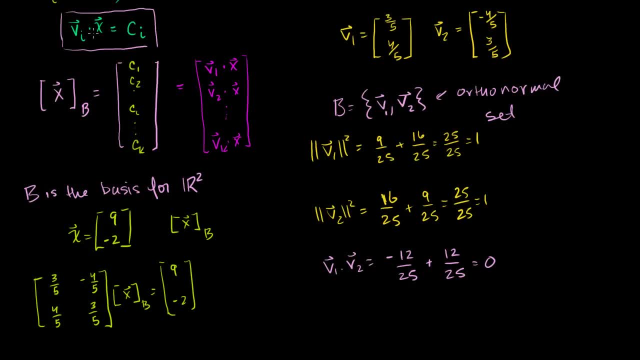 And in the 2 by 2 case it's not so bad. But we have this neat tool here for orthonormal sets or orthonormal bases. So instead of solving this equation, we can just say that x, represented in b-coordinates, is going to be equal to let. 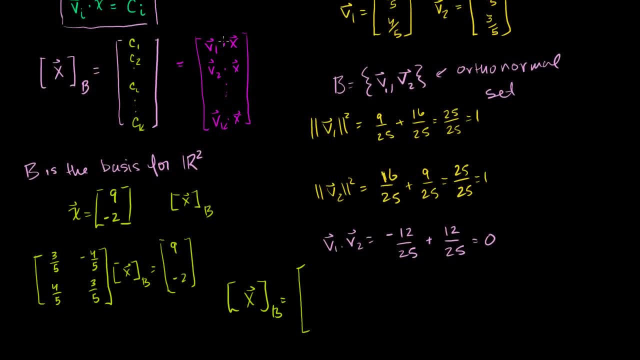 me scroll down a little bit. it's going to be equal to v1,, which is this guy right here dotted with x. So it's going to be v1 dot x, And then this guy right here is just going to be v2 dot x. 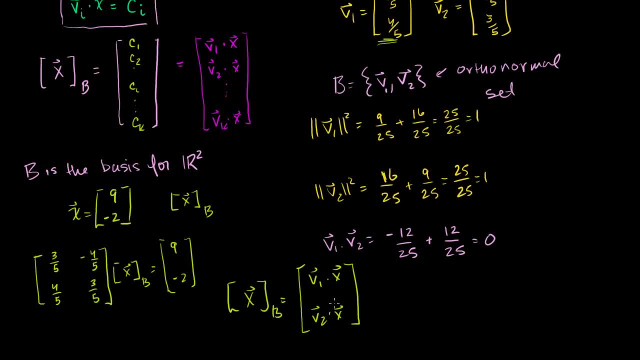 And I can do this because this is an orthonormal basis. And what is this? equal to x is 9 minus 2.. If I dot that with v1, I get 9 times 3 fifths, which is 27. 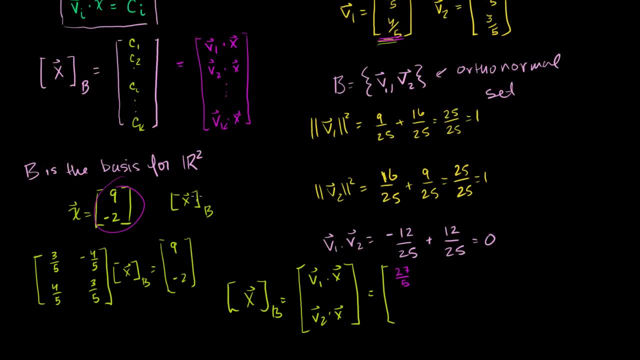 fifths right, 27 over 5.. 9 times 3 is 27 over 5, plus minus 2 times 4 fifths, So that's minus 2.. Minus 8 fifths right, Minus 2 times 4 fifths is minus 8 fifths. 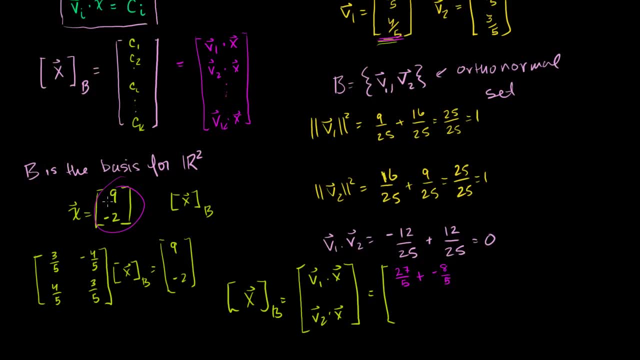 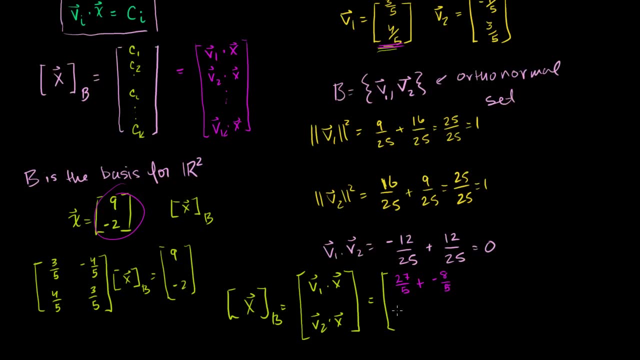 And then the second term is v2 dot x. So v2 dot x, I get 9 times- let me scroll up a little bit- 9 times minus 4 fifths, That's minus 36 over 5, plus minus 2 times 3 fifths. 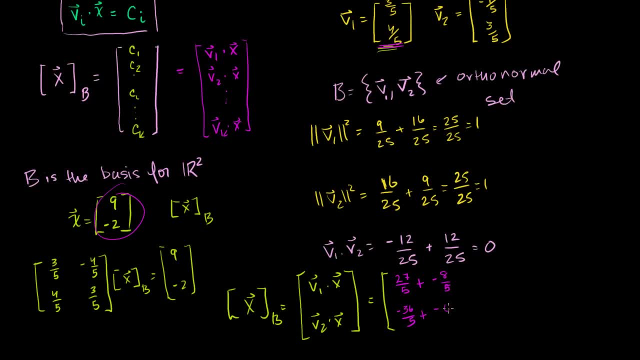 So that's plus minus 2 times 3 fifths, is minus 6 fifths. So the b-coordinate representation of x- just being able to use this property right here of orthonormal bases, is equal to what is this: 27 minus 8 is 19 over 5.. 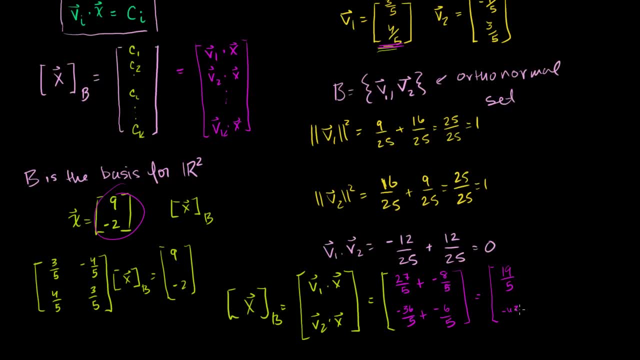 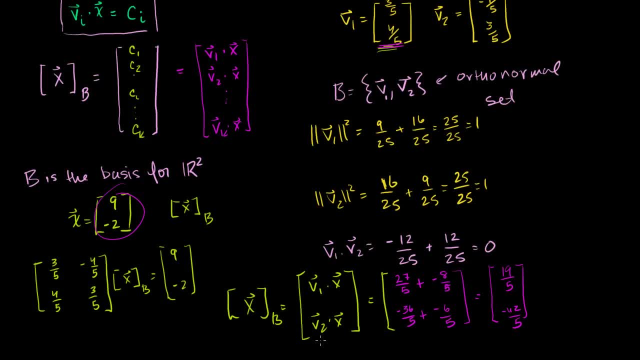 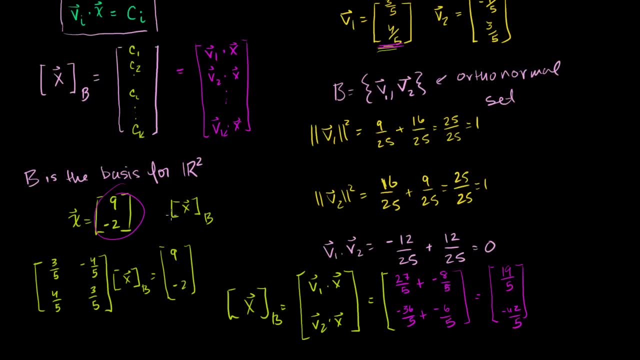 respect to that basis becomes a lot easier. This is just an example in R2.. You can imagine how difficult could it be if you start dealing with R4 or R100.. They're all of a sudden solving these systems aren't so easy. 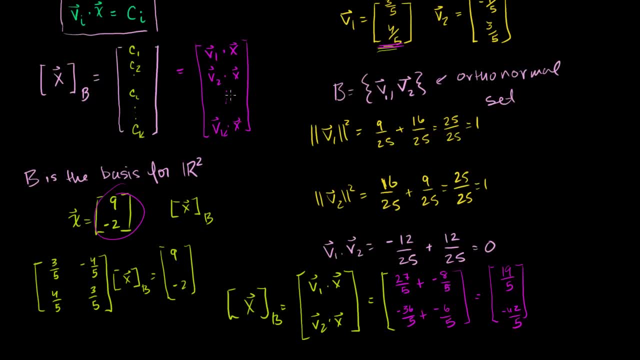 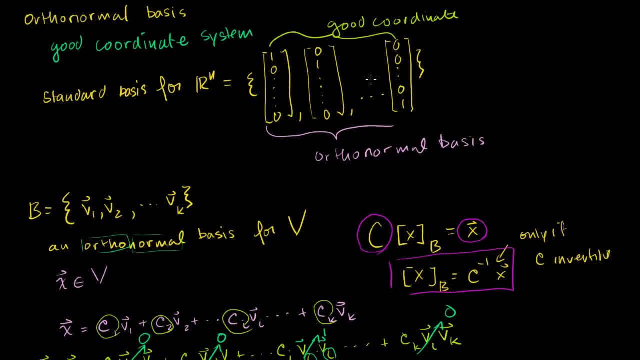 But taking dot products here are always fairly straightforward. So earlier in this video, when I said orthonormal bases, what are they good for? I said: will the standard bases is good, that these are good coordinate systems. We've used it before.